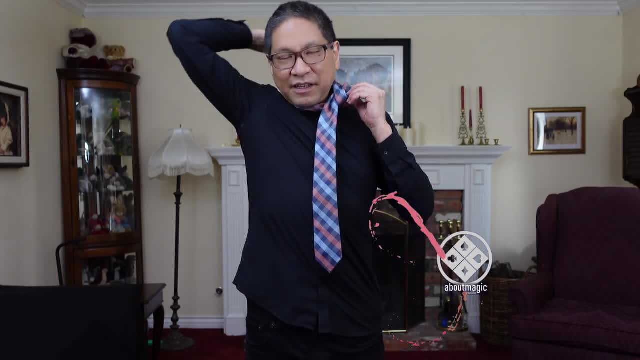 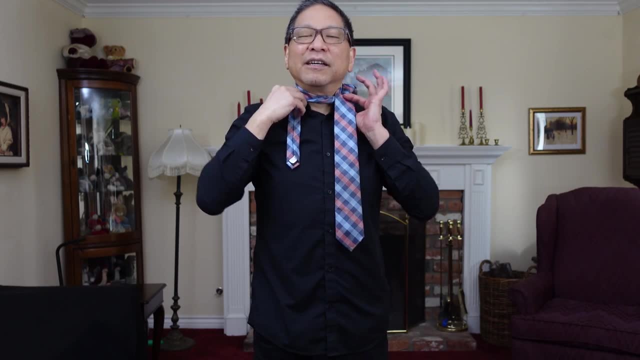 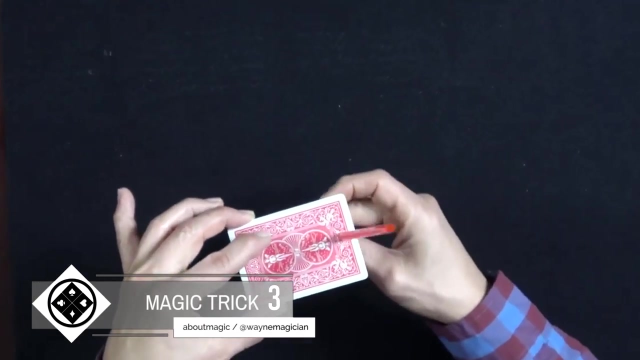 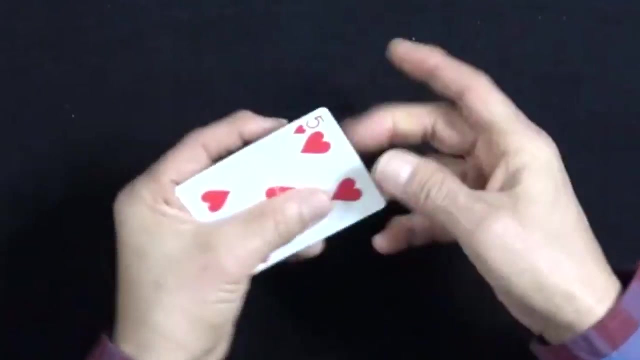 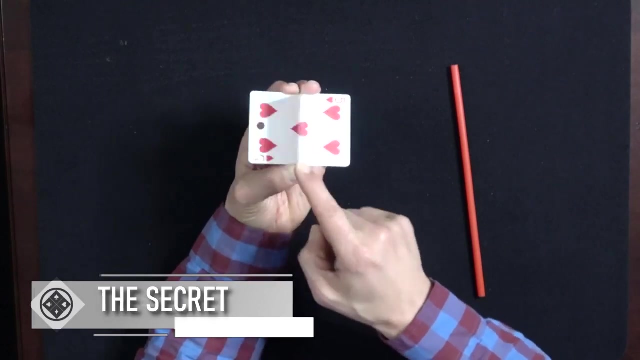 material inside of the other end. Now it looks as if I've wrapped the tie around my neck, but all I have to do is pull and it comes undone. But you create this flap. So the first card has a hole punched in it at the top and this right. 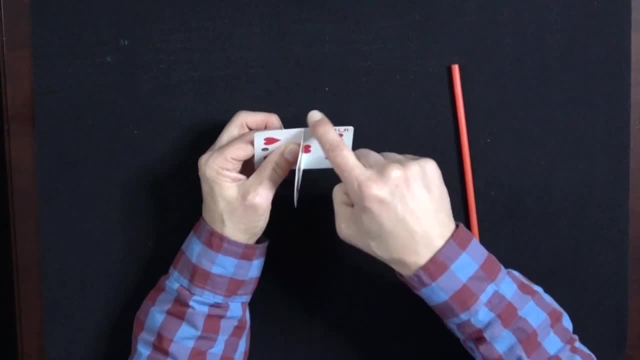 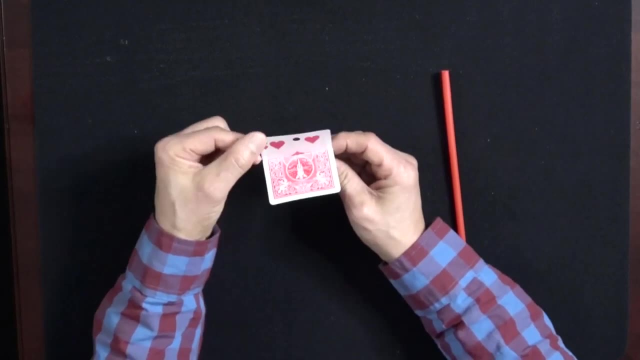 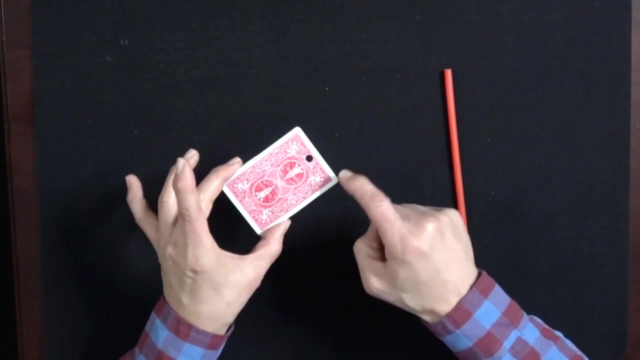 here is the second card that's glued onto the first card with the half down here. So it's two cards thick on this side, Single card here and a single card here. So you start out showing the hole. Actually you can do it in reverse, but I like showing the hole. 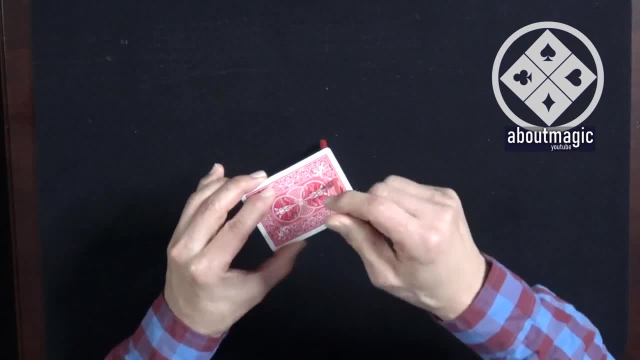 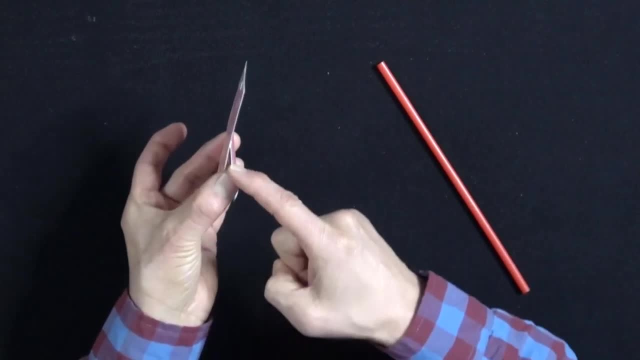 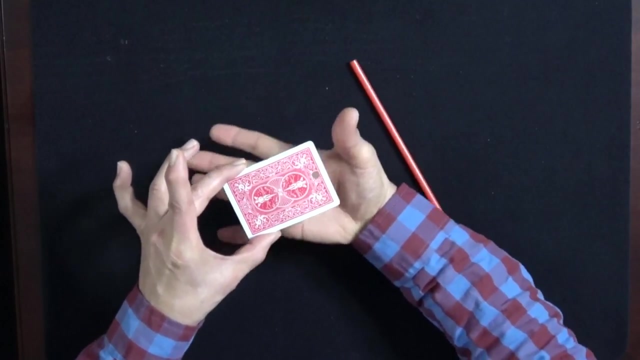 And, just so happens, a straw fits through this hole. punched hole here. Now, the way I'm holding it on the back side is I'm actually letting it hang down just a little bit, and that way it makes it easy. so when I want to turn the card over, I take my fingers and I actually flip it over as I. 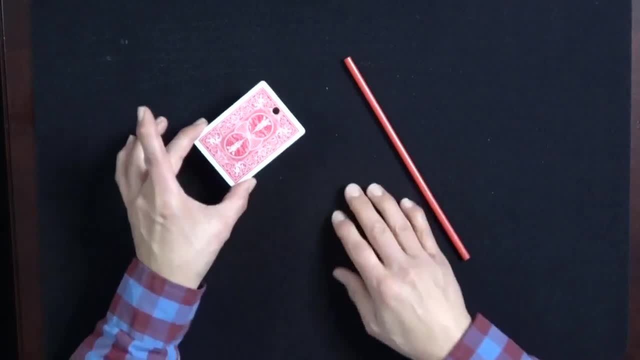 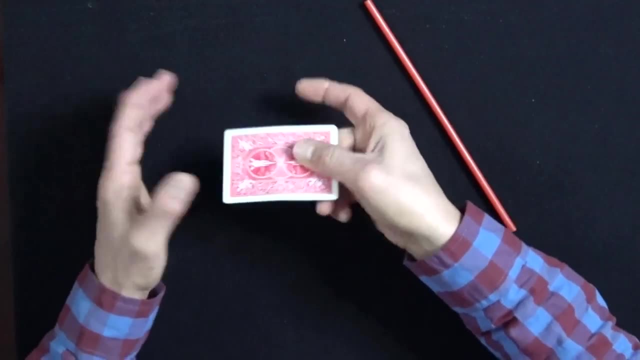 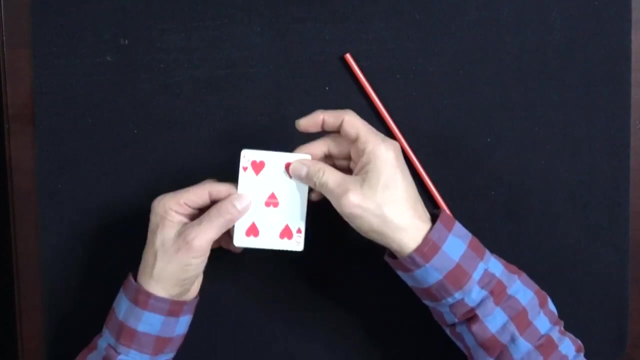 turn over the card. So the way I did it in the presentation is just like this. Again, from the side It looks like this: So yeah, turn it over. and yes, there is a little bit of a line here. You can kind of cover it with your fingers. 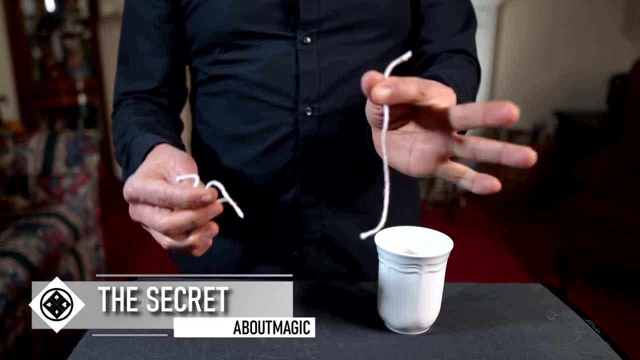 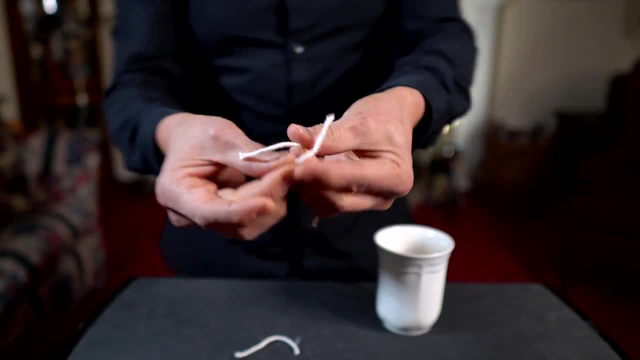 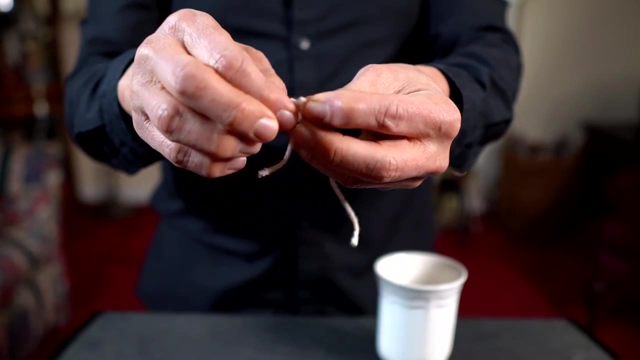 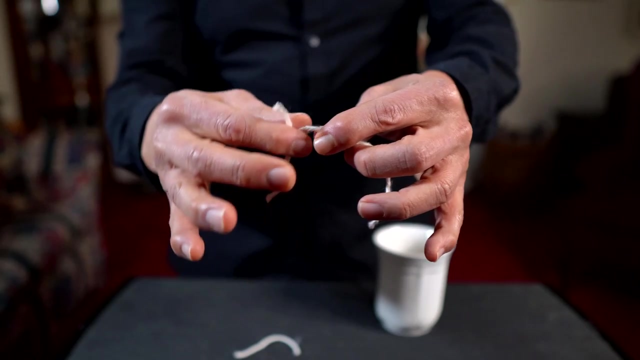 You're going to need one length of string, two smaller lengths of string, and all you're doing is tying these short lengths on the longer ones. I'm going to tie this one here. Don't tie it too tight, but don't tie it loose enough that it falls. but you want a knot on there that slides, and we'll do. 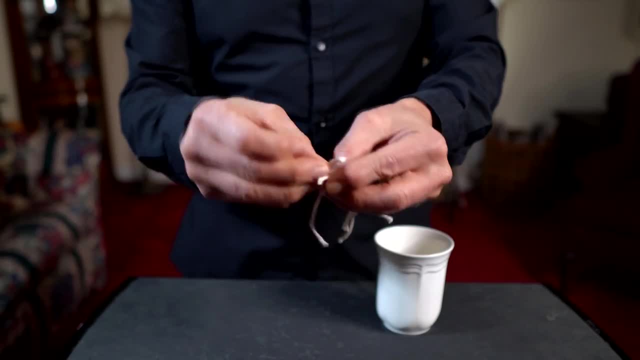 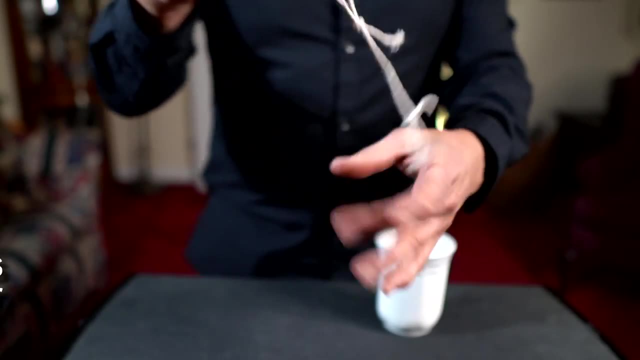 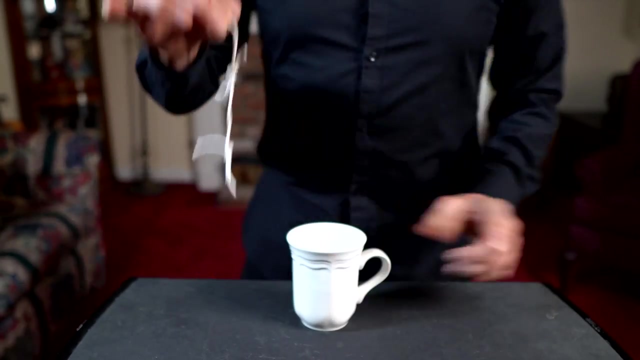 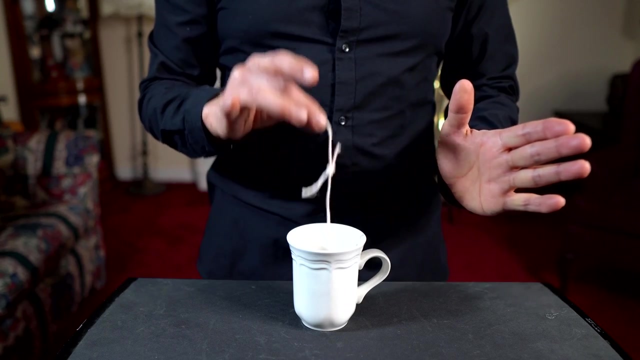 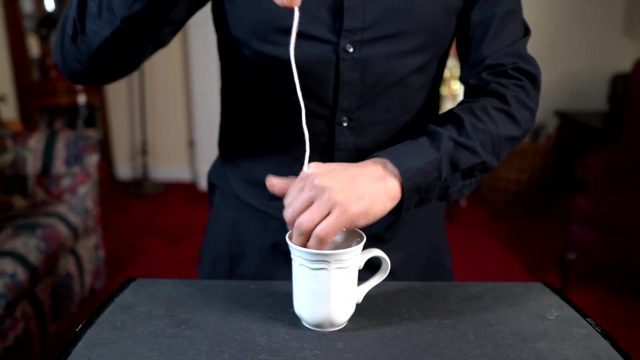 that one more time here. That looks, for all practical purposes, like three strings that you've tied together. All you do is take your strings, bring it out, show it and then take your hand, place it in to the cup and then, as you pull up, you slide the string through the hole. 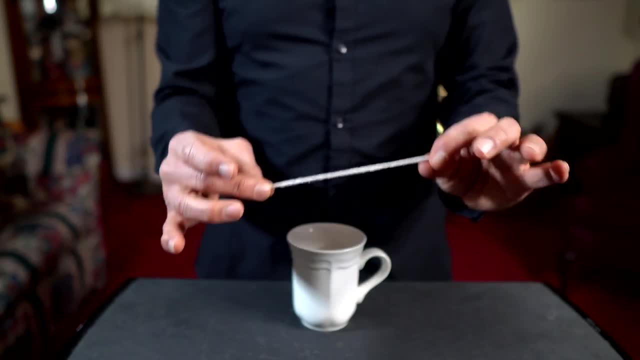 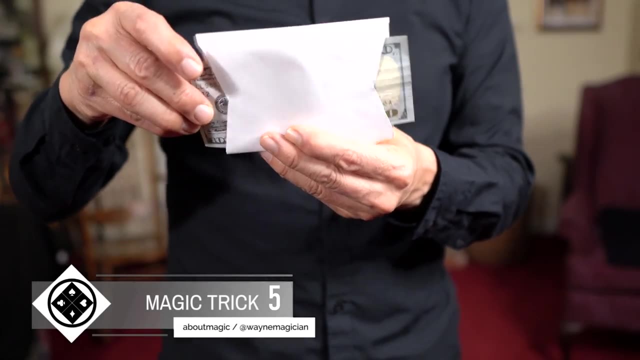 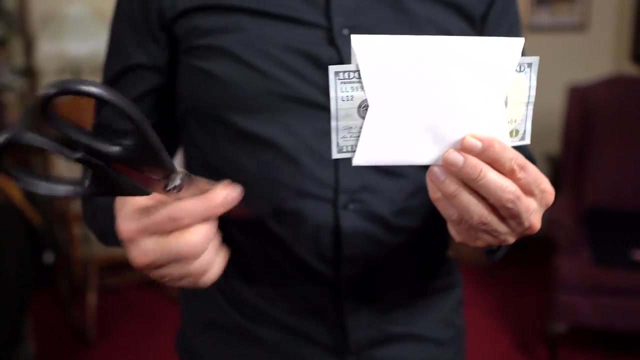 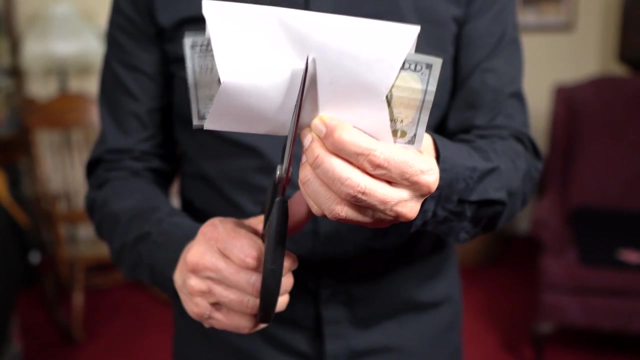 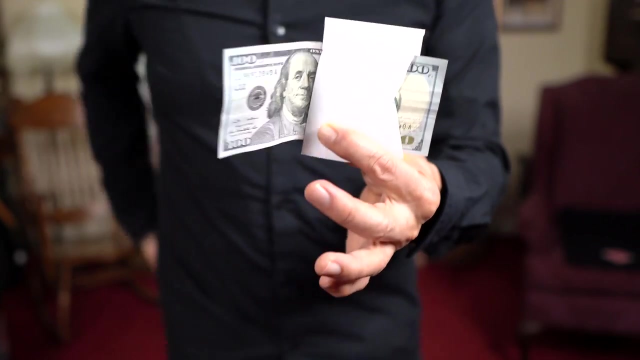 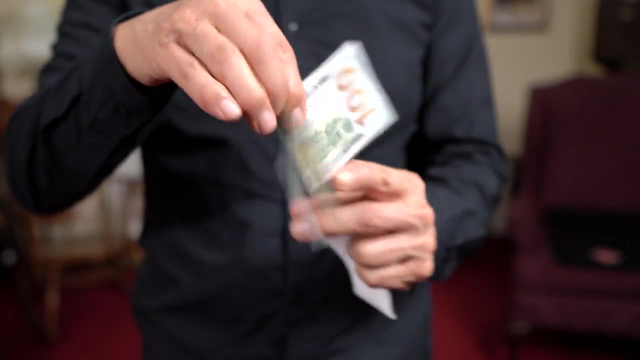 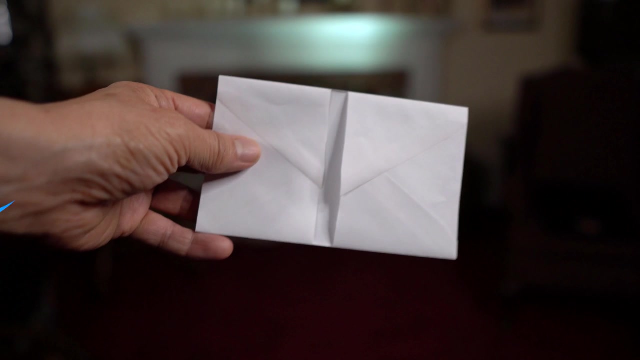 Slide the strings off of the rope, Slide the knots off the string, So that doesn't do much work. There you go. Yeah, Good luck everyone. Thanks for watching. I'll see you guys next time. See you, Bye, bye. Thank you, Thank you. 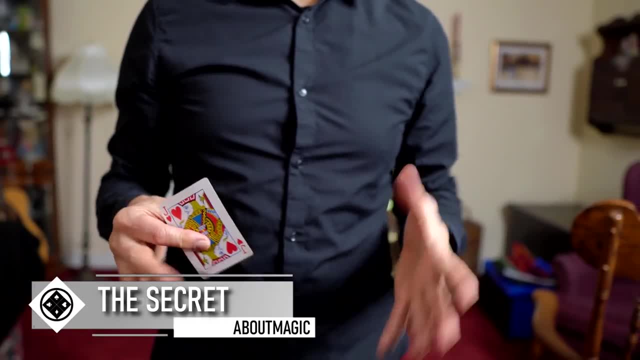 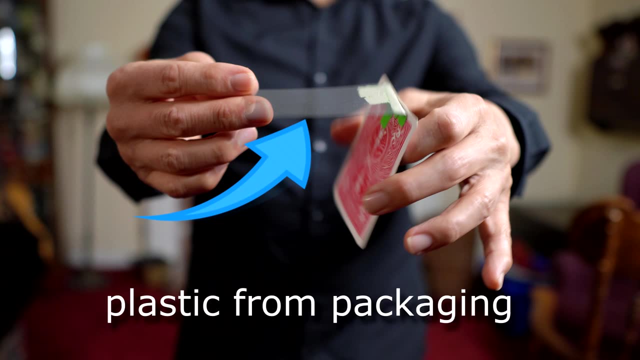 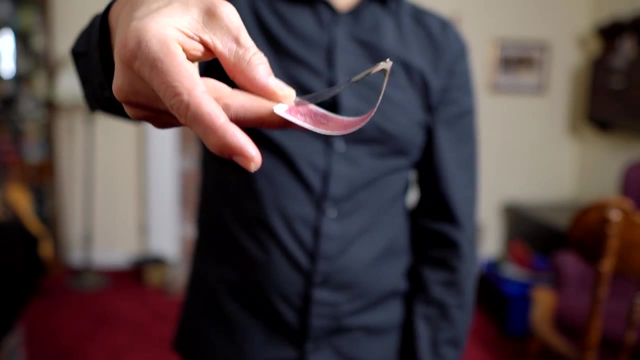 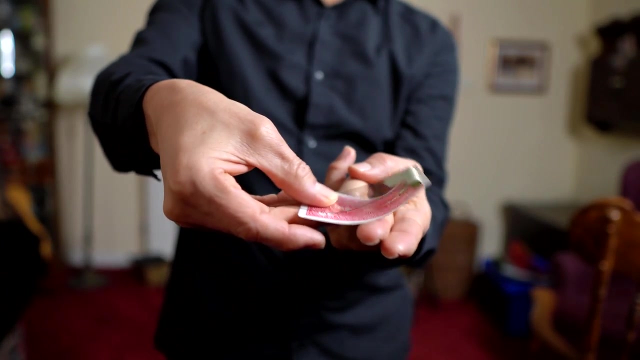 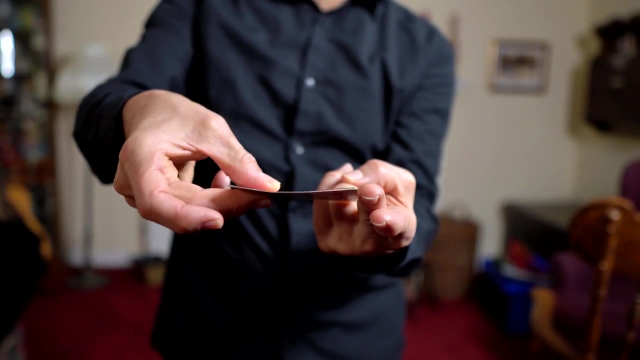 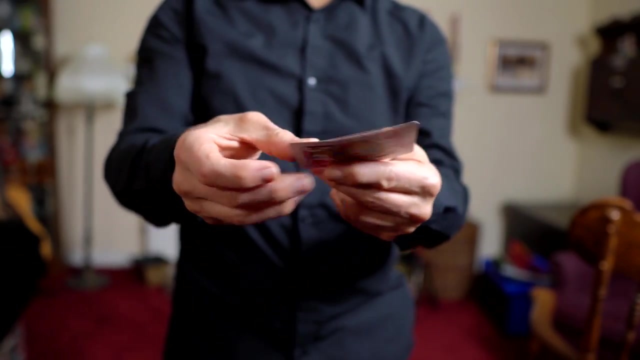 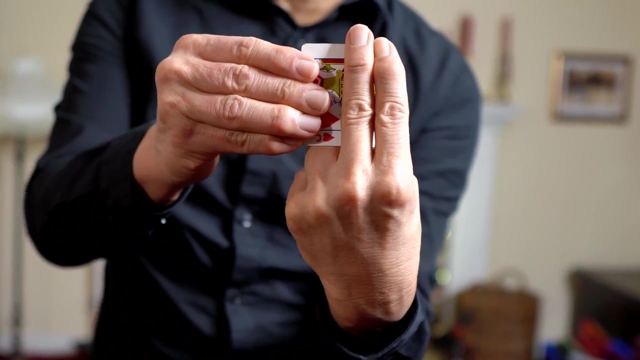 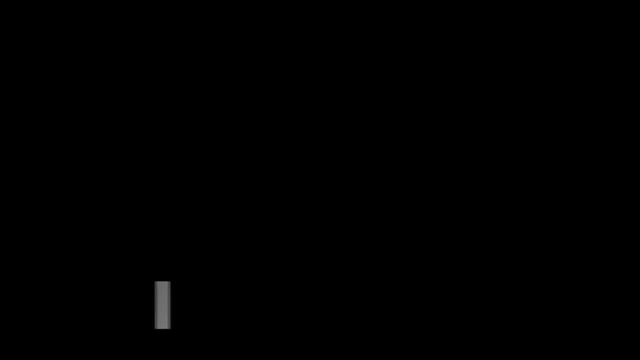 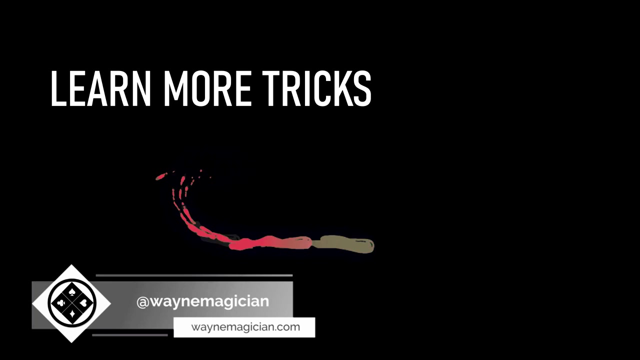 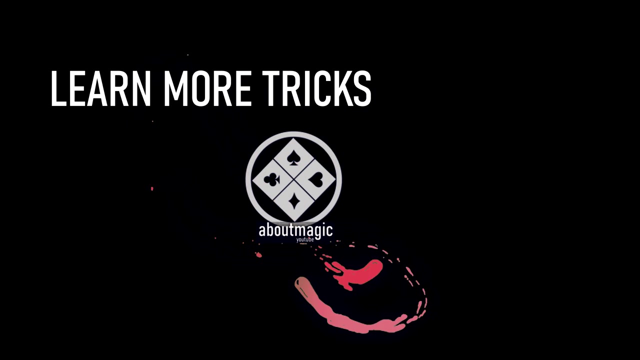